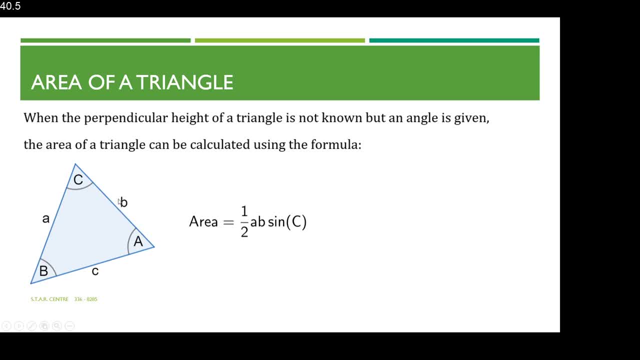 For angle B, the side opposite, that would be the side B, and for angle C, the side opposite, that would be the side C, And this applies to all the triangles, as we go on. And also to point out that, in any formula, the common letters represent the lengths of the sides and the capital letters represent 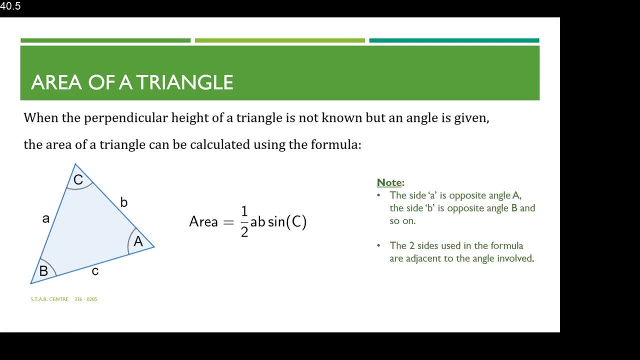 the angles And also for this formula. the angle that is given the two sides that's involved in the formula are the two sides that's adjacent to that angle. That means the two sides that are touching the angle. So if we have sine C, this is the angle that's given. The two sides that's touching that angle here would be A and B. 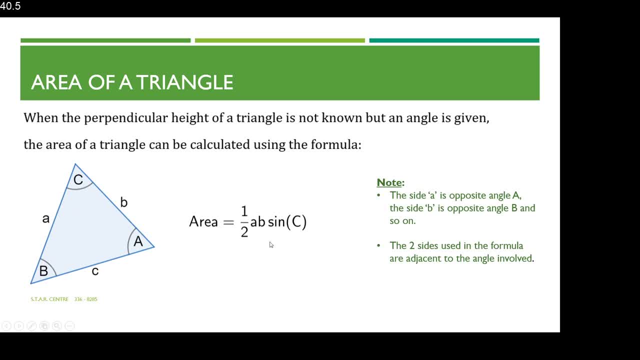 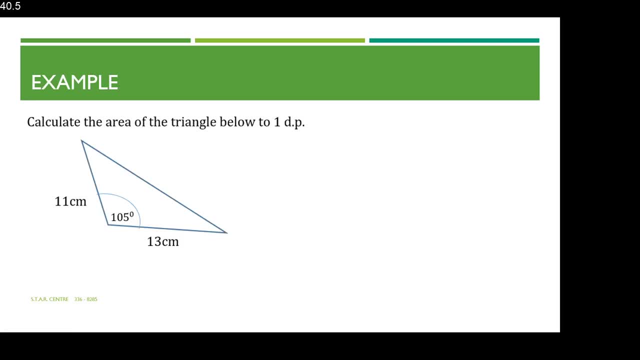 So in any formula for area of a triangle using this you would have the two sides that's adjacent to the angle that is given Example. calculate the area of the triangle below to one decimal place. So area of a triangle equal a half A, B, sine C. 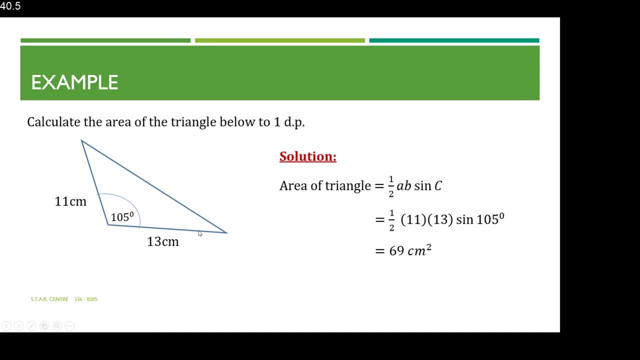 So this is our angle and the two sides that are adjacent to that angle. So just substituting into our formula, we would have a half multiplied by 11, multiplied by 13, multiplied by sine 105 degrees, And just putting all of this into the calculator would give us 69 centimeters squared and 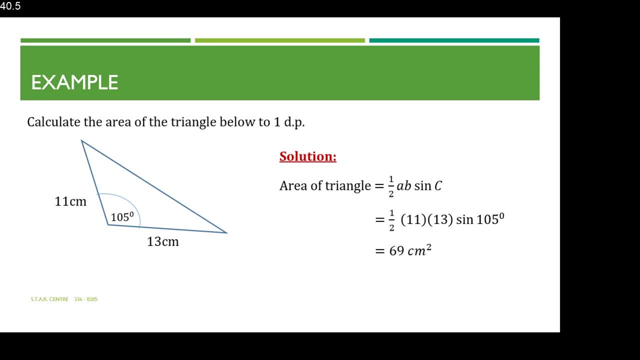 just another thing to point out would be that when we are working any of the trig functions in our calculator, it's important what mode the calculator is in, because it does affect the answer. So for c-sec mathematics your calculator should be in degrees mode. 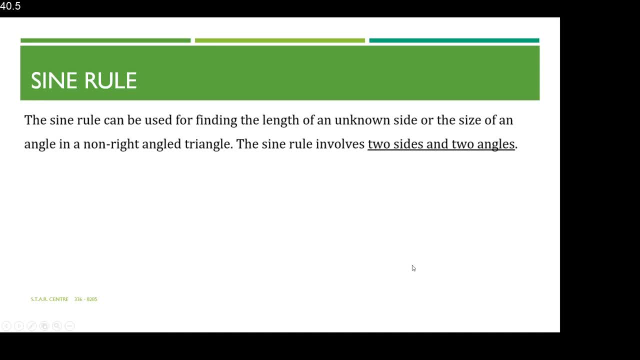 Sine rule. The sine rule can be used for finding the length of an unknown side in a triangle or the size of an angle in a triangle. that is se style, not a right angle triangle, or it could also apply for right angle triangles Now in the past, when we 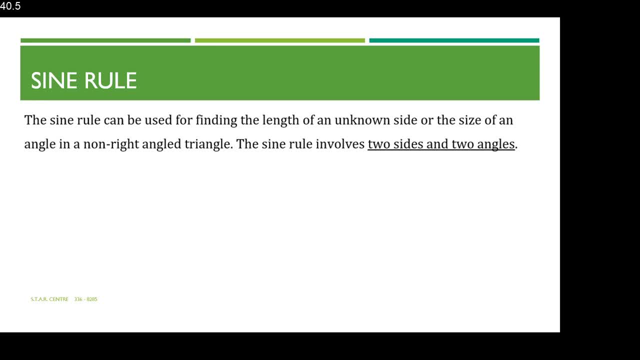 had to find the length of a side or an angle in a right angle triangle, we could. we use Pythagoras theorem and we use the trig ratios according to what we needed to find and what information was given. However, if we have triangles, that is, that are non-right angle triangles and we are required, 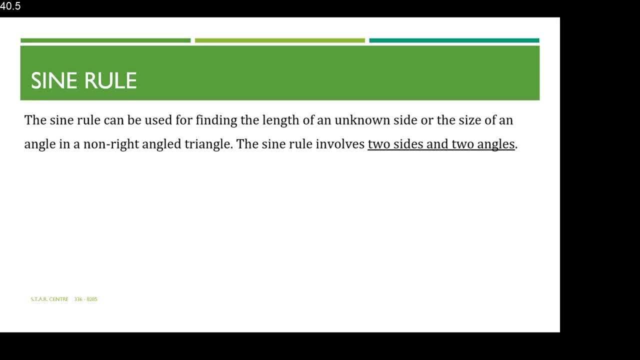 to find the length of a side or the size of an angle, then we can use this rule called the sine rule, and the sine rule involves two sides and two angles, and again this can work for both right angle and non-right angle triangles, but specifically used for non-right angle triangles as it's. 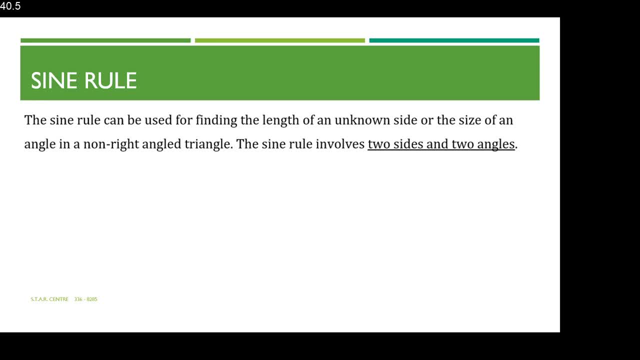 simpler to use Pythagoras and trig ratios for the right angle triangles. So the sine rule looks like this: we have a over sine a, equal b over sine b, equal c over sine a, And from our triangle, if you look at it, it's very similar to the one that we did for area. 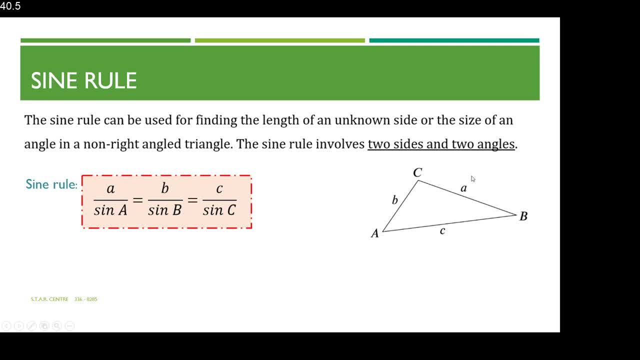 where the angle a, the side opposite, that is, a side e, and for angle b, the side opposite, that is, angle, is side b, and for angle c, the side opposite, that is side c. And at any point in time, only two out of the three parts here would be relevant for our calculations, as you would see. 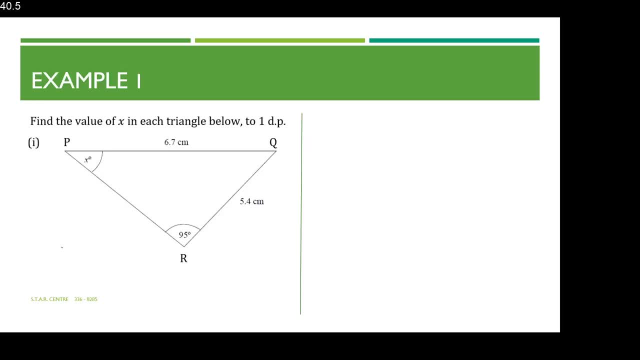 in the examples. Example one, find the value of x in each triangle below to one decimal place. So part one, this is our angle x. we have triangle PQR. So this is angle P. this is a side opposite. so this would be the side P. Here is. 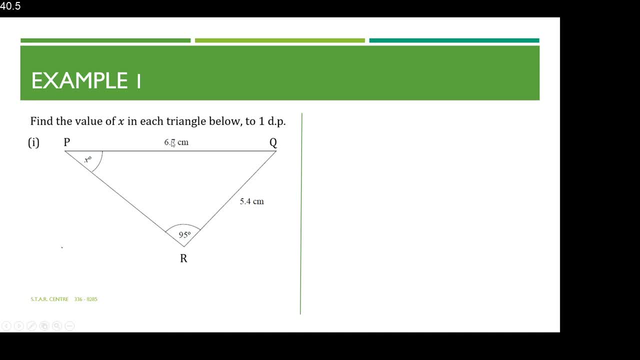 angle R, the side opposite. that would be the side R. Now we do not have angle Q and we do not know the side opposite, Q, so therefore, for our sine rule, the letters that are relevant, the sides that are relevant, would be P and R. We cannot use Q because you don't have the information. 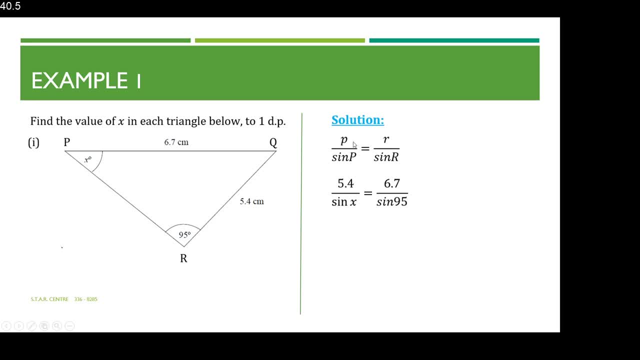 relevant for Q. So we will use P over sine P, equal R over sine R. and just a reminder that the common letters represent the lengths of the sides and the capital letters represent the angles. So P would be the side P, which is 5.4.. Sine P will be sine of x. R is the side opposite. 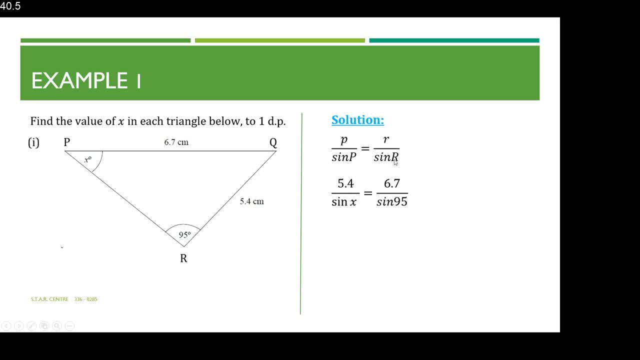 angle Angle R, which is 6.7, and sine R will be sine of 95. So it gives us 5.4 over sine x equals 6.7 over sine 95. From this point we are going to cross, multiply and that will give us 6.7 by sine x, by. 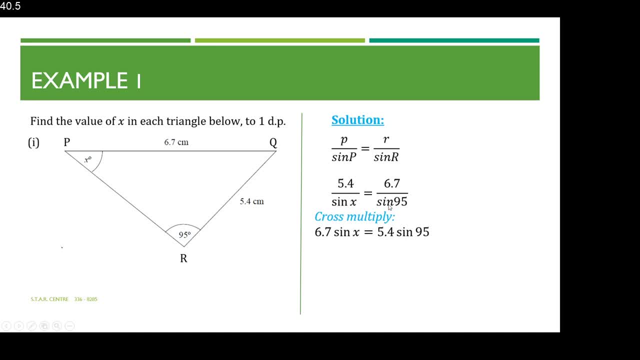 equal 5.4 by sine 95. Making sine x the subject of the formula would give us 5.4 sine 95 over 6.7.. I have chosen to leave this. leave it in this form, as when we work it out and we round off. 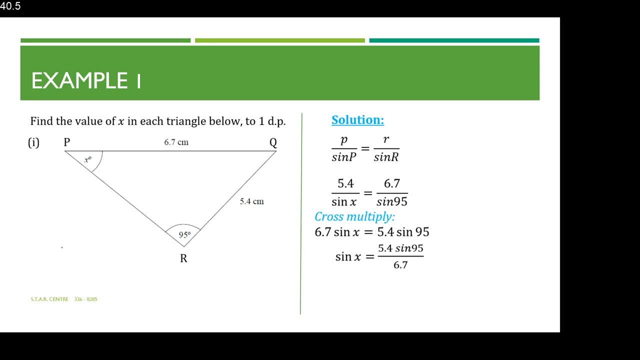 rounding off too much can affect our the accuracy of our answer, So I'm leaving it in this form. and to find x we have to take the inverse. so x is equal to sine inverse of this. putting it all into the calculator, using brackets as well, This will give us: x is equal to 53.4 degrees and I am rounding off to 1.. That is 1.5. 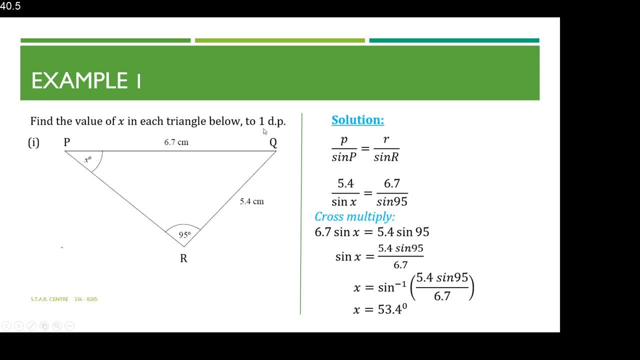 That is 5.4. place, because the question specified to one decimal place. If it did not specify, then you could round it off to the nearest degree or however you like, but once it's specified in a question you would need to follow the instruction. 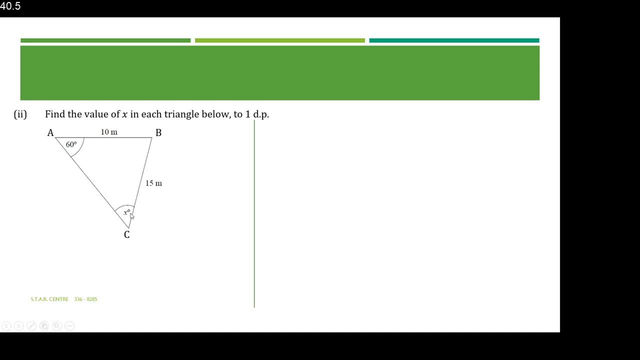 Part 2, find the value of X in this triangle. So, looking at it, we can see that we have angle A and then the side opposite A. I have angle C involved and the side opposite C We have nothing. for B, no information. so therefore, our sign: 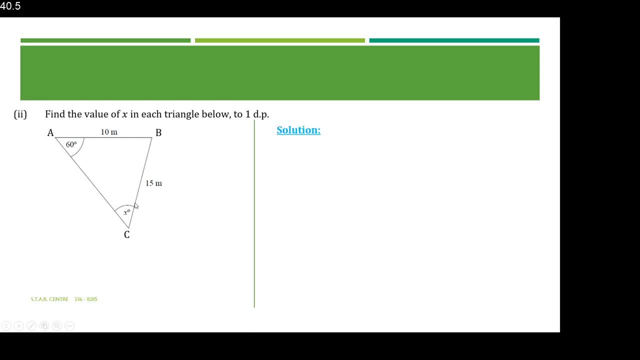 rule in this case would involve A and C. Now for the sign rule. it doesn't matter whether we put the C on the left hand side and the A on the right hand side, or vice versa. The A could be on the left and the C could be on the right. we would 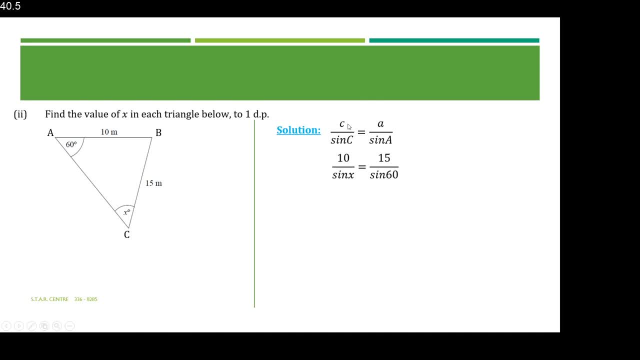 get the same result. So using C and A, we'll have C over sine C, equal A over sine E and getting our value from the diagram. This common letter C represents the side opposite angle C, which is 10.. Sine C would be sine of X. equal A, Common A would be the side. 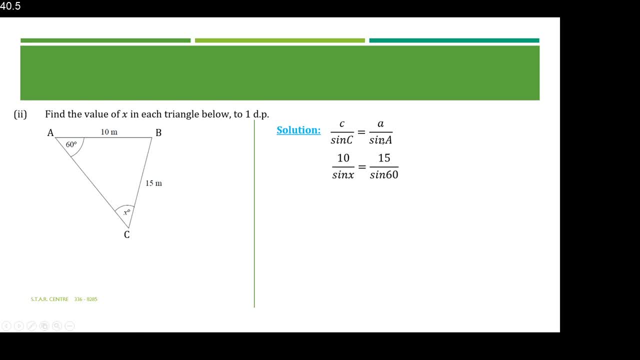 opposite, that angle A, which is 15, and sine A would be sine of 60. From this point we are going to cross multiply, which will give 15 sine X equal 10 by sine 60. We want to make X the subject of the. 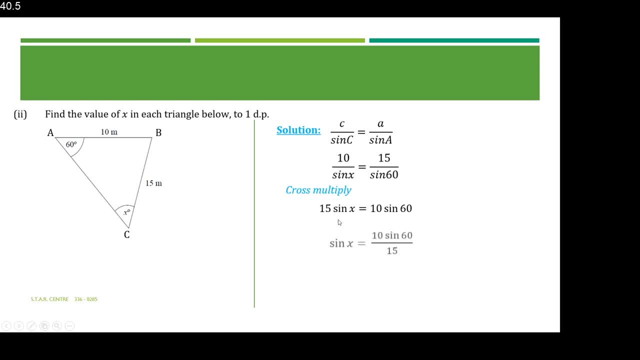 formula. So for now I'm just going to have sine X here, and on the right hand side we'll have 10 sine 60 over 15, and to get X we would take the inverse, which will give us 35.3 degrees to one decimal place. Example 2, find the length of the. 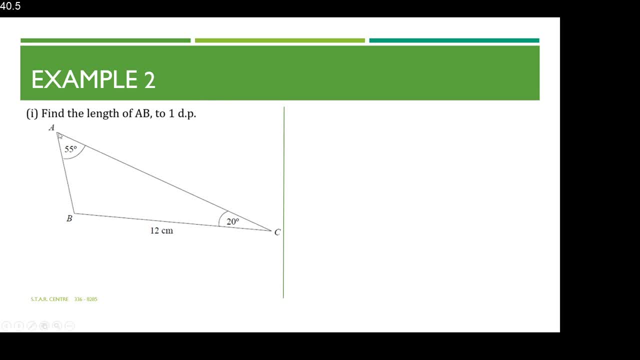 side AB to one decimal place. So this question is similar to the previous ones. The difference is, however, that we are finding the length of a side now instead of an angle, So we are given two angles and the side, and we need to find another side. So, as stated earlier, the 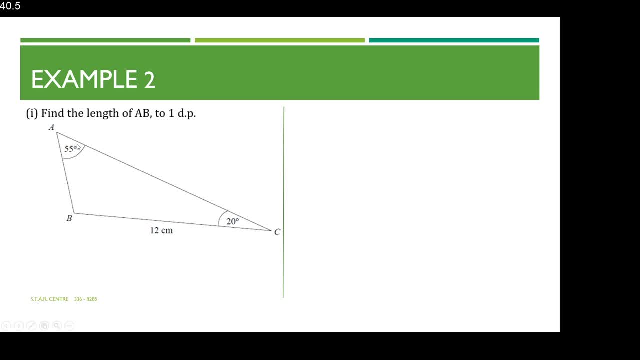 sine rule involves two angles and two sides. So we have the angle A, the side opposite that angle, which is which will be the side A. I have angle C and I want to find the length of AB, which is this side, and this is the side that's. 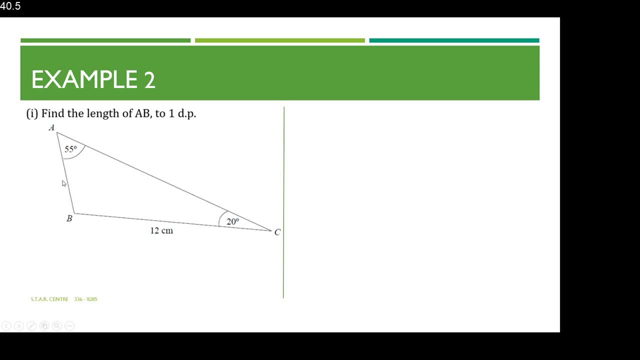 opposite the angle C. So in our sine rule we would have the letters A and and C involved. So C over sine C is equal to A over sine A, Substituting our values. the common C is this side, which is AB over sine 20, that's sine C equal A, which is: 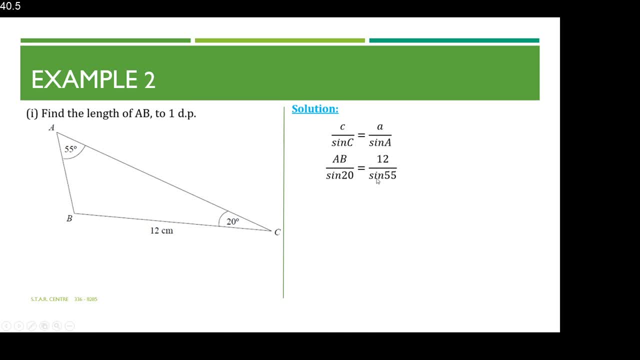 the side opposite angle A, that's 12, and sine of A would be sine 55. Cross multiplying would give us AB by sine 55 equal 12 by sine 20.. And we want to make AB the subject of the formula, which would give us AB equal 12 sine 20 over sine 55, and that will give 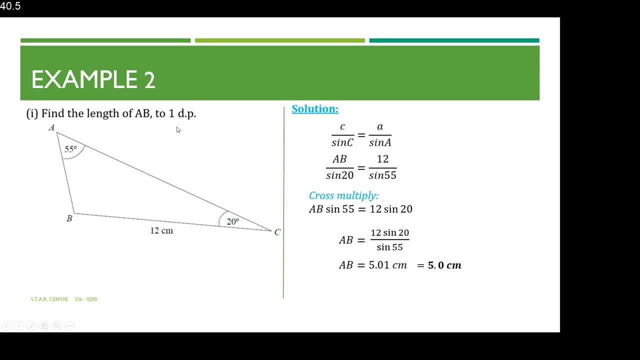 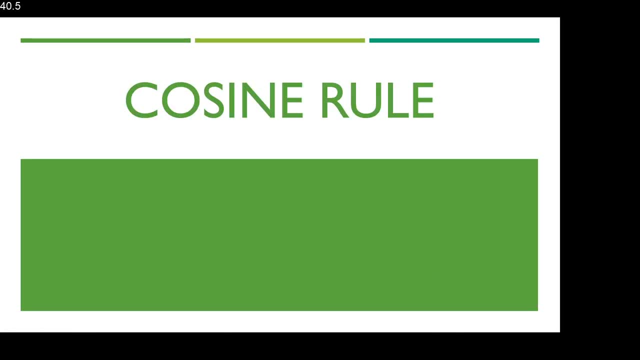 us 5.01 centimeters, And since the question specified to one decimal place, I would write that as 5.0 centimeters. Okay, now we are going to look at the cosine rule. The cosine rule is the cosine of A over sine A, So we are going to look at the cosine rule of A. 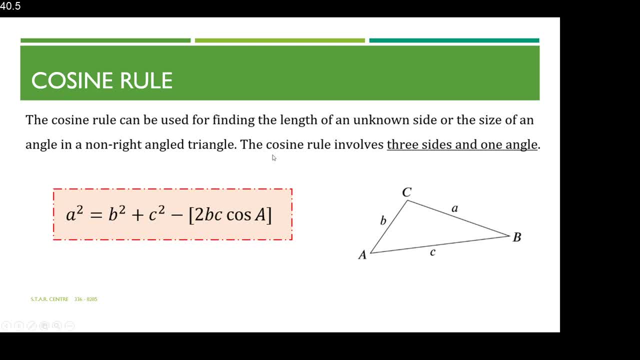 over sine A, So the cosine rule can be used for finding the length of an unknown side or the size of an angle in a non-right angle triangle. So so far the information is the same as sine rule. However, the difference is that the cosine rule involves three sides. 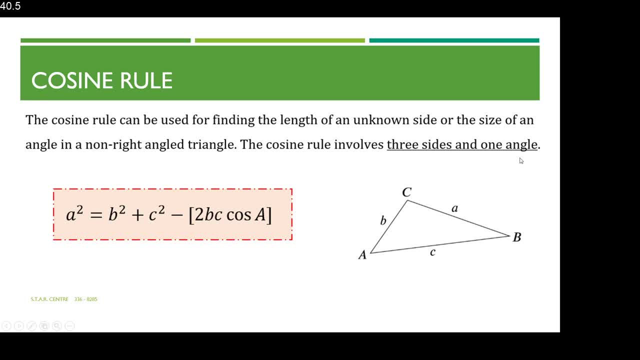 and one angle. So, in comparison, the sine rule involves two sides and two angles. The cosine rule involves three sides and one angle. So it's also important, moving forward, that we know the difference and we need to know which is the correct formula. So we are going. 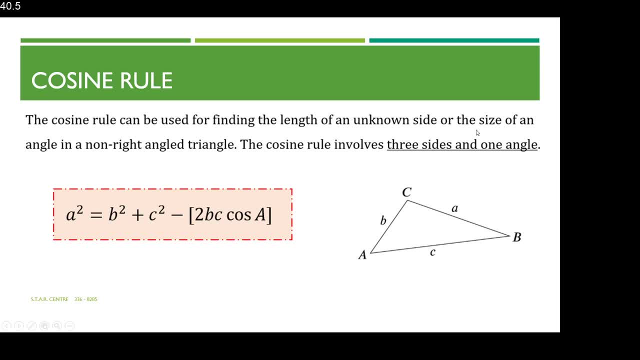 to use the cosine rule. The cosine rule involves two sides and two angles, So it's also important, moving forward, that we know the difference and we need to know which is the correct formula. To figure out which is the correct formula, it's based on just this part here: the information. 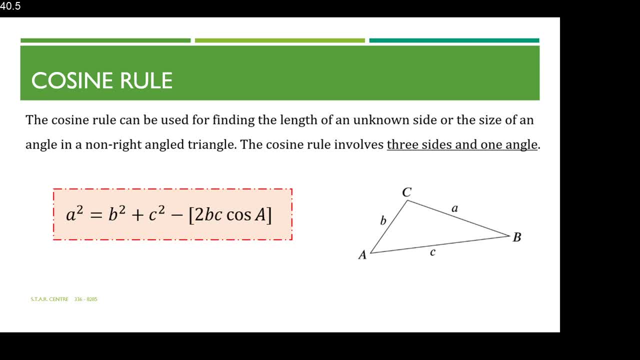 that is given. So in a triangle, whether we want to find the length of a side and an angle, if we have two sides and two angles involved, it's the sine rule, But if we have three sides and one angle involved in the question, it's the cosine rule. 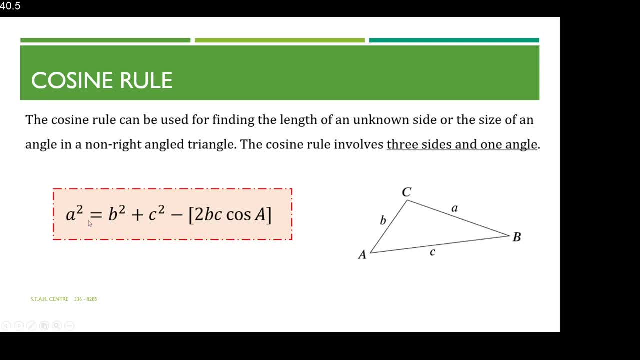 So the cosine rule would be: A squared equal, B squared plus C squared minus 2, BC cos A, a and a, b and c are variables. that means it can be any other letter. we can have p, q and r and any other letter given. so in this triangle, just as before, we see that if this is angle a. 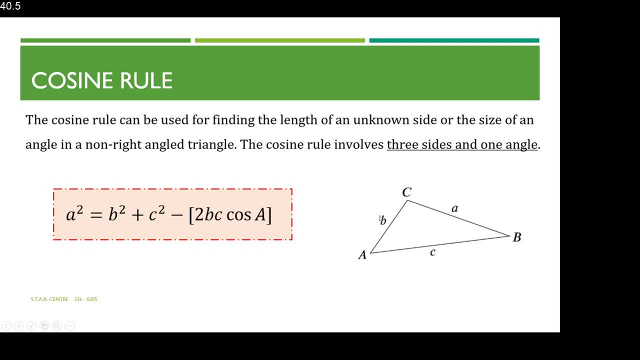 side a is opposite that. if this is angle b, side b is opposite that and so on. for this formula, i would like to point out that the letter that i have on the left hand side of the equation, which is a, corresponds to the angle in that cosine rule, so cos of a. so whatever letter or angle we have, 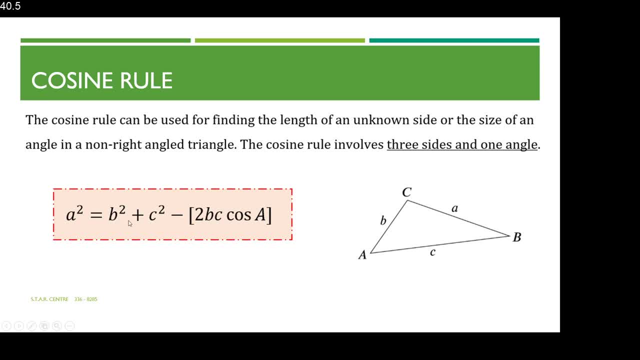 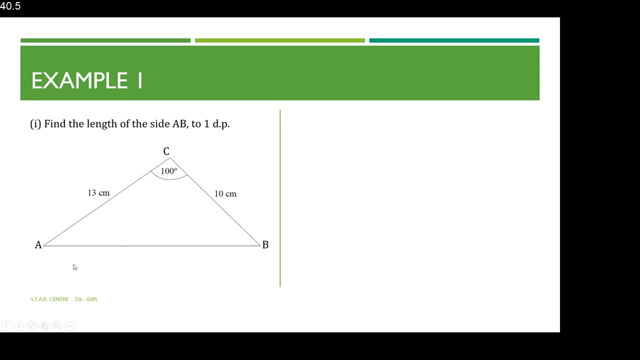 here corresponds to this side, and this in between would just be the other two sides, in any order: b and c or c and b. so let's see how the cosine rule is used. example one: find the length of the side a, b to one decimal place. so the side a, b is this side and we can see. 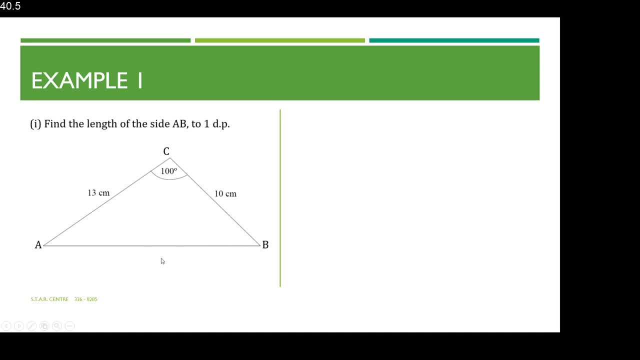 that the side a- b is this side and we can see that the side a- b is this side and we can see that this side is opposite the angle c. so that means we have the cosine rule and even though i have triangle a, b and c, because our angle is 100 degrees, our cosine rule letters would be written: 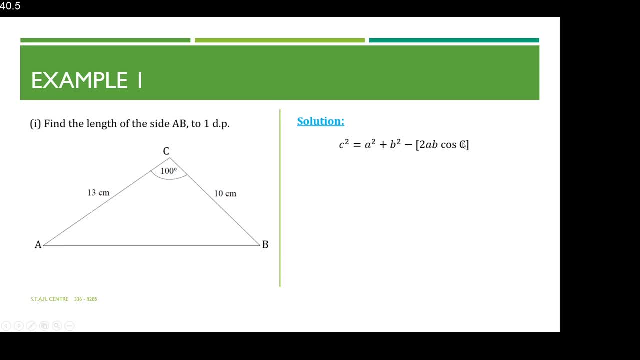 slightly different in terms of: if this is the angle c, then here would also be c. this is the side c, substituting those values. so c squared, that's the side we want to find. so that's a, b squared, a squared. a is the side opposite angle a, which is 10, b squared, is the side opposite angle. 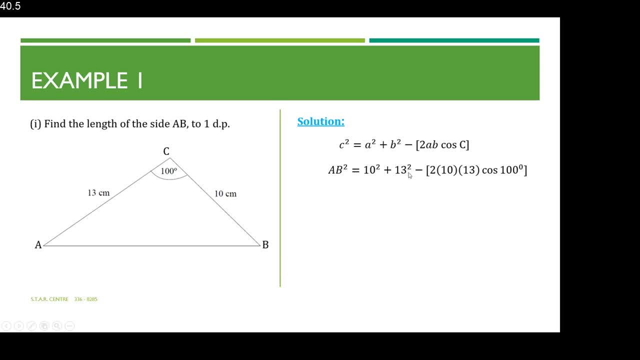 b, which is 13. so we have 10 squared plus 13 squared, minus open brackets: 2 a, which is 10, by b, which is 13, cos of c and the angle c, there is 100 degrees. all right, so working that out this part of it, 10 squared plus 13 squared will give us 269 in brackets. 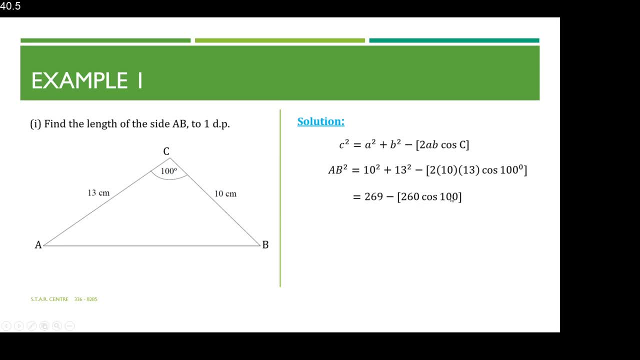 this part of it: 10 squared plus 13 squared will give us 269 in brackets. the 2 by 10 by 13 will give us 260 by cos 100.. it's important to work out brackets first. it's not 269, take away 260. we have to work out the brackets first and then subtract. 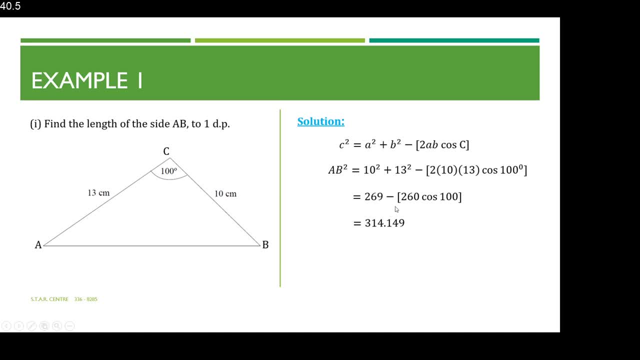 so putting this into the calculator, 269 minus open bracket, 260 cos 100 close bracket, this gives us 314.149. but notice that this is equivalent to a- b squared. we just need to side a- b, so therefore a b would be the square roots of that, which gives us 17.7. 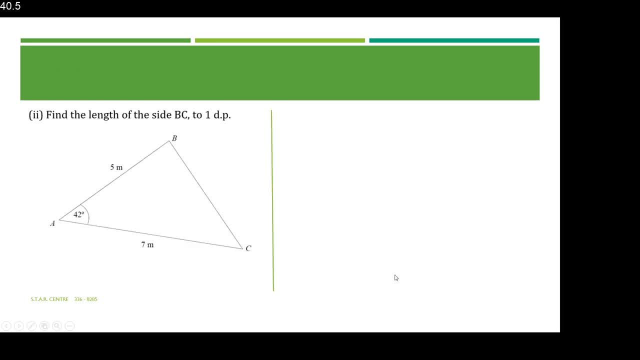 centimeters to one decimal place. part two: find the length of the side b c to one decimal place. so b, c is the side opposite e. so this is the side a, angle e. then this is the side c and the sides b. so we are going to use the cosine rule. 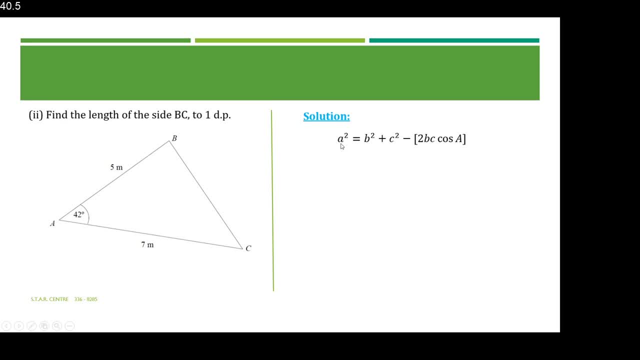 since we are looking at angle a, the letter that i have on the left hand side is also a, so a squared equal b squared plus c. squared minus 2: b c cos e, so a squared would be what we want to find, so i'm leaving that as it is. b squared is the side opposite b, so that's 7 squared. 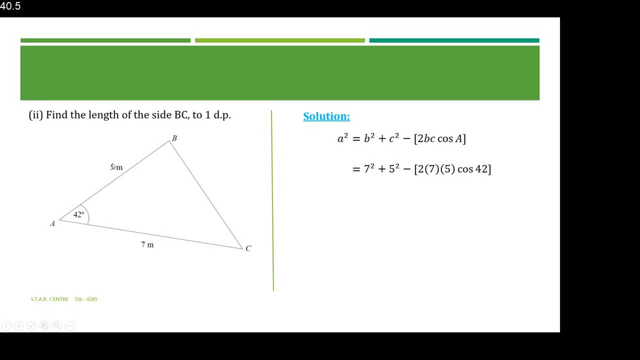 c squared would be the side opposite c. c is the side opposite angle c, so c squared would be 5 minus 2 b c cos of a, so that's cos of 42 degrees. so 7 squared plus 5 squared gives us 74, and in the brackets, 2 by 7 by 5 will give us 70, and in the calculator i'm putting, putting in: 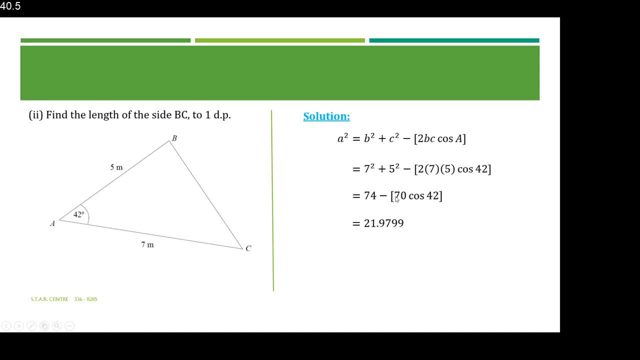 our values exactly as shown: 74 minus open bracket, 70 cos 42 close brackets. so brackets, they are important and that gives us 21 point nine seven, and this is the value of a squared. so get a. i need to take the square roots of that, which gives 4.7 centimeters. example 2: find the size of an angle x to one. 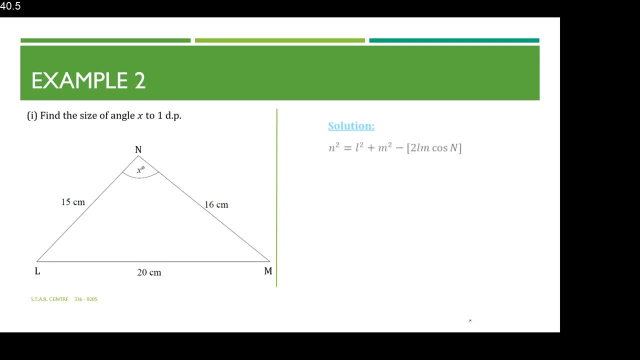 decimal place. so our solution: from our diagram we see that we have angle n, x, angle n and the side opposite, that is, 20.. so since the angle that is involved would be n, Then in our cosine rule on the right hand side we have cos of n. 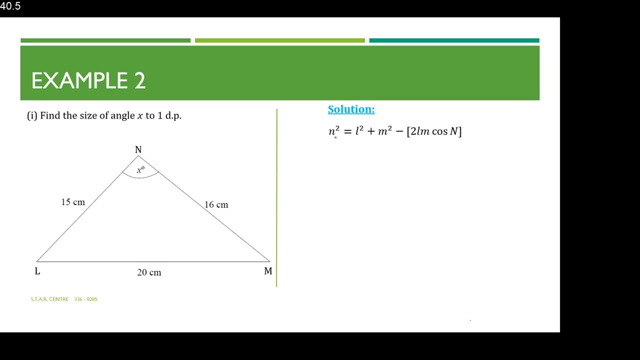 which means on the left hand side we have n squared. So n squared is equal to l squared plus m squared minus 2 lm cos of n. So substituting those values, let's just identify what those values would be. So angle n would be x. Our side n would be. 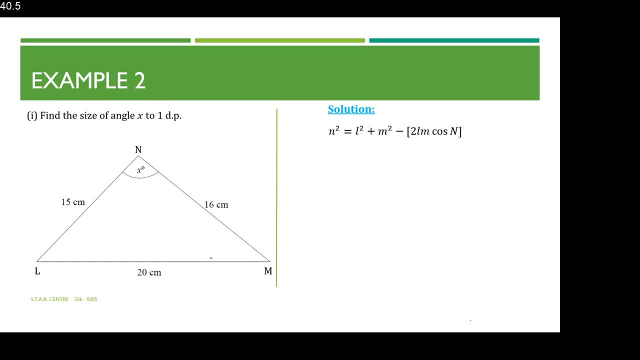 opposite, angle n, which is 20.. Then we have angle m, The side opposite, that is 15, and 16 is the side l. So substituting those values we would have: 20 squared is equal to 16 squared plus 15 squared minus 2 by 16. 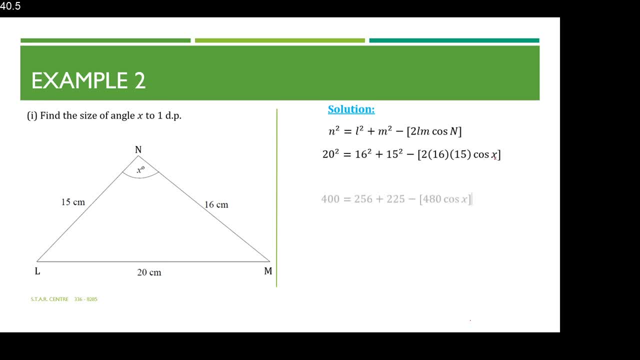 by 15 cos of x. Simplifying 20 squared would be 400.. 16 squared is 256.. 15 squared is 225 minus and, in brackets, 2 by 16 by 15 gives 480 and this remains as cos x. And just simplifying these two values here. 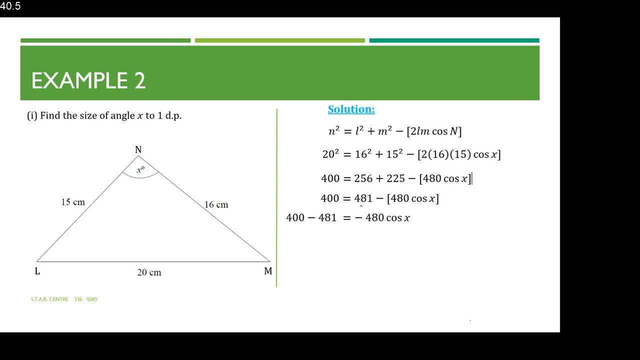 256 plus 225 to give the 481, and then I'm going to solve for x. So we are going to do that step by step. So now on the left hand side we'll have 400 minus 481 is equal to, and we are left with. 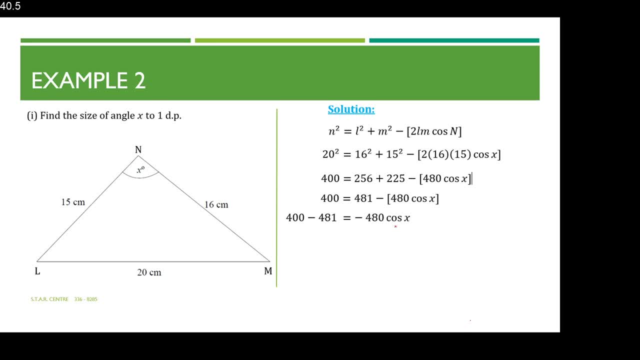 this part of it: minus 480, cos x. So this on the left hand side simplifies to give minus 81. So you have: minus 81 divided by minus 480 is equal to cos x. So from this point to solve for x we'll need to take the inverse. 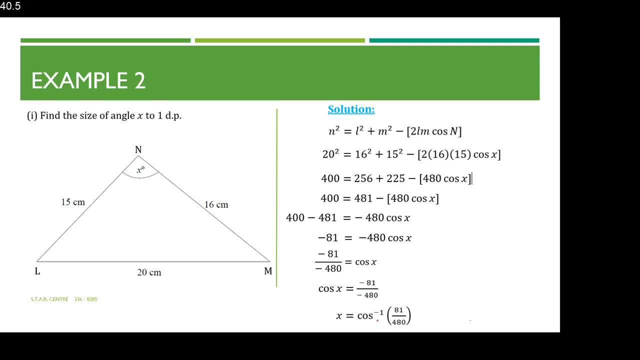 So therefore, x is equal to cos inverse of 81 over 480. minus 81 over minus 480 is the same as 81 over 480. Which is equal to 80.3 degrees to one decimal place. Part 2: find the size of angle A. 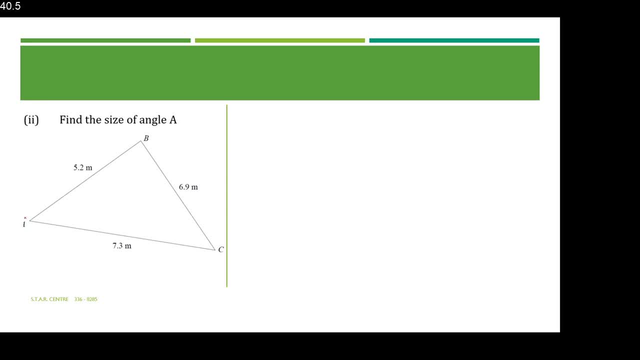 So this is supposed to be angle A. It's not shown clearly on the diagram, So this is angle A. That means that in our cosine rule we will have A squared on the left hand side, So A squared is equal to B squared plus C squared. 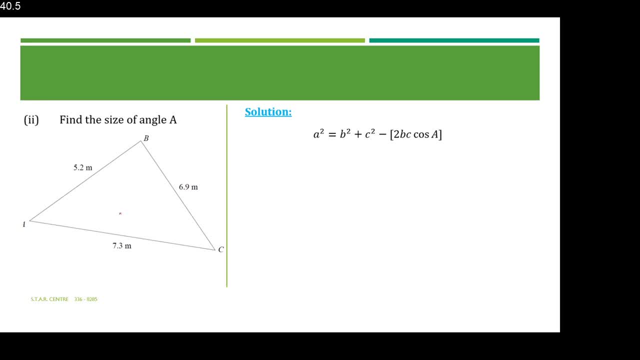 minus 2B squared In that respect. so that's going to give like 6.9c cos. So those here are going to be 4.9c cos. C squared would be the side opposite angle A, which is 6.9 squared. 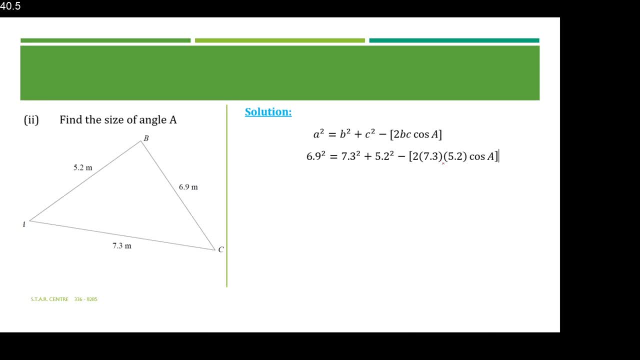 b squaredB is the side opposite angle B, which is 7.3, and so that will be 7.3 squared, And C is the side opposite angle C, which is 5.2.. So 5.2 squared minus 2 by 7.3, by 5.2 cos of B. 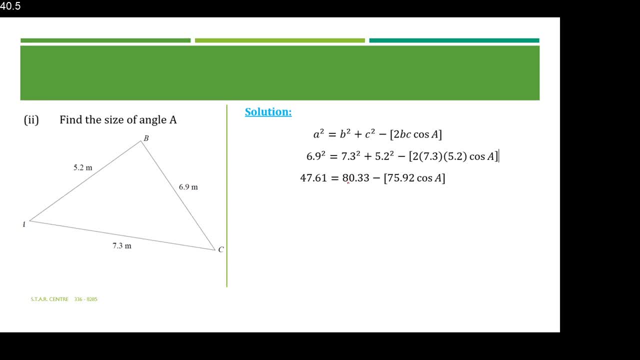 47.61 equal. adding these values would give 80.33, and working out this in brackets, the 2 by 7.3 by 5.2 gives 75.92 and we have cos a. so i'm solving for a one step at a time, so we'll have 47.61.